into places and cities And at the heart of that is just how we can really help the infrastructure as well, as what's calling for change and the role and potential that has come in the infrastructure So that will be used to work with people, and how we can really help people. 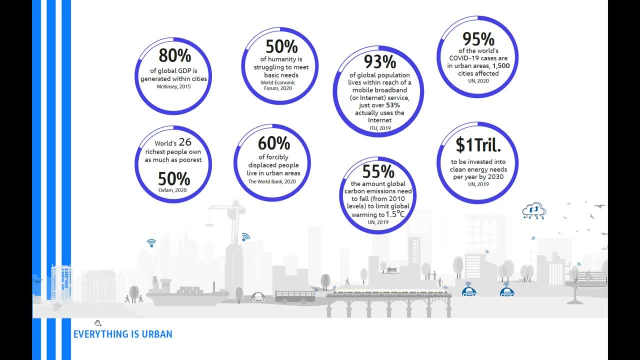 of that really are the challenges that we're facing day to day in in society and globally, and some of these statistics which we use to illustrate the challenges we face include a lot of those around the growth of cities, around how cities are predicted to to grow and become. 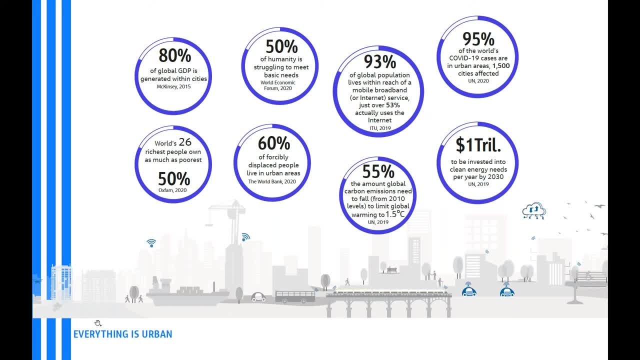 more and more dominant in the future, but also disparities. so in the bottom left, how the world's 26 richest people in as much as the poorest 50 in the whole world, which really is kind of opens your eyes in terms of not only how the world is growing but how the world is separating and 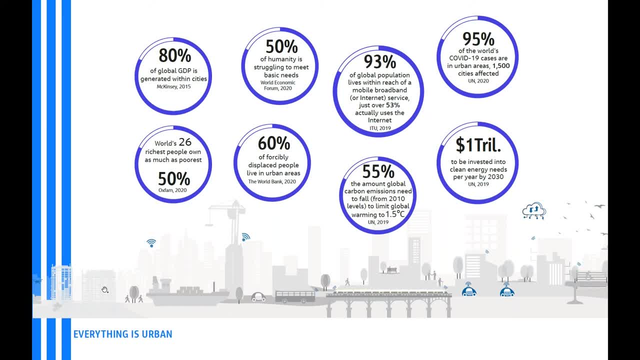 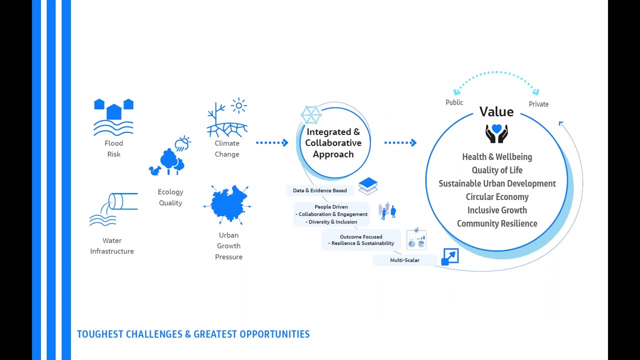 and how people are losing out. so as we go forward, we'll illustrate some ways which we're trying to use our projects really to benefit society as a whole. and this slide really moves on from that previous one into how do we take the incredibly tough challenges on the left hand side, particularly around climate. 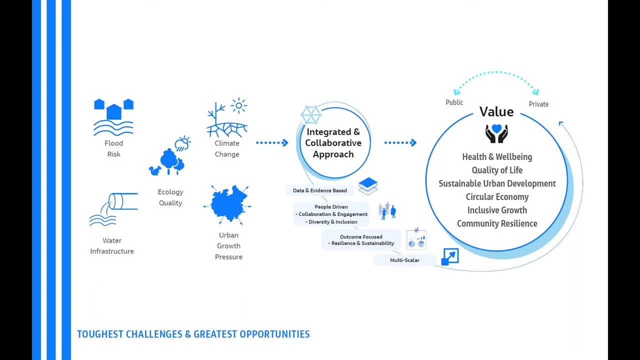 around all forms of resilience in society and within the environment, and how do we translate those challenges spatially into projects? and really we believe in a completely integrated collaborative approach and, as you see, under the the circle in the middle, we use data. everything we do is evidence-based and about layering data, we collaborate. 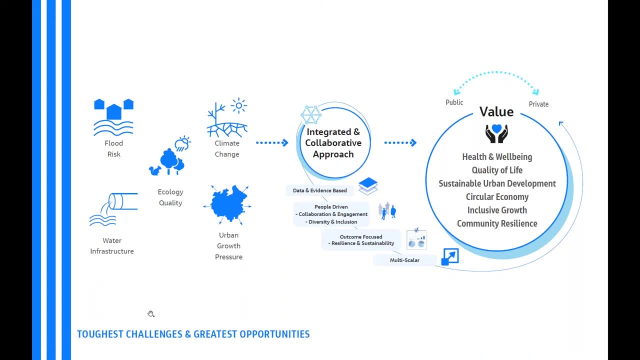 we want to engage, we want to work closely with with the public, with stakeholders, with clients, and our focus is really on on resilience and sustainability as a key driver and we believe in a multi-stellar approach. so working regional, regional scale, down to neighborhood, down to site-specific scale and in terms of output, really we're focused on delivering. 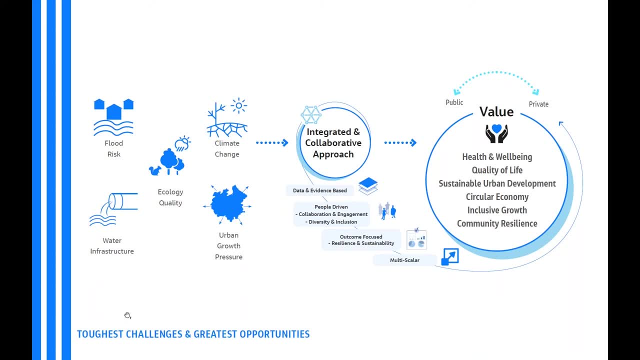 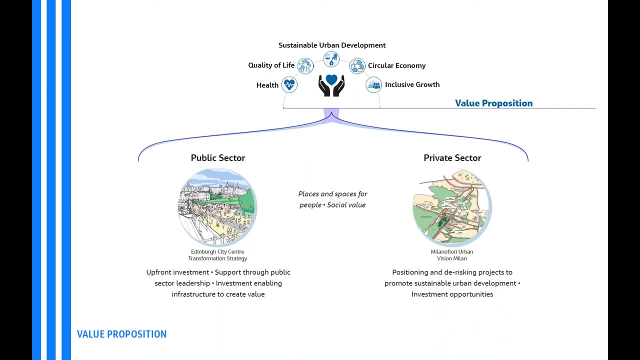 projects that improve health and well-being, quality of life, sustainable. they promote circular economy, inclusive growth and around community resilience. and in terms of of how that can happen, we see very much. the partnership between the public sector and the private sector is absolutely crucial to this and, as jacobs, we have the 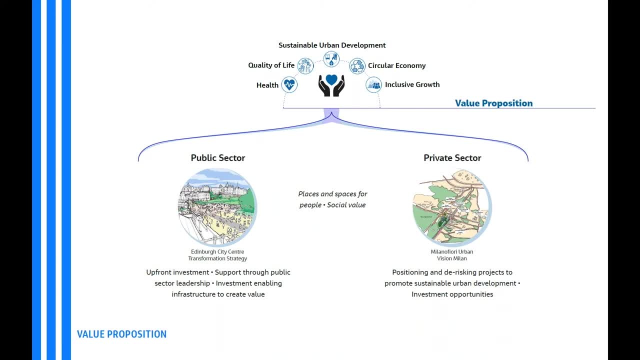 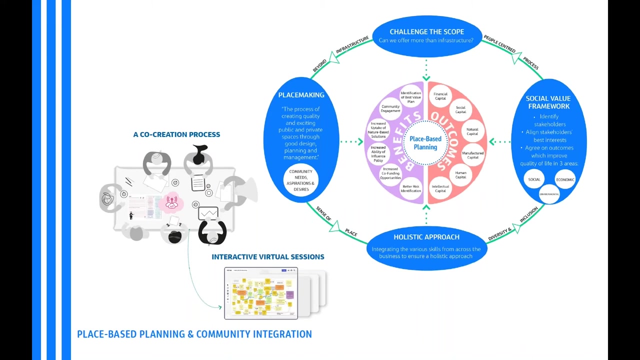 benefit of working in both camps and very much wanting to help, be the facilitator to bring them together, and we see public and private collaboration really as the only way to deliver the against these tough, toughest challenges which we've illustrated in previous slides. so we have been working with other teams in jacobs and trying to develop this holistic approach. 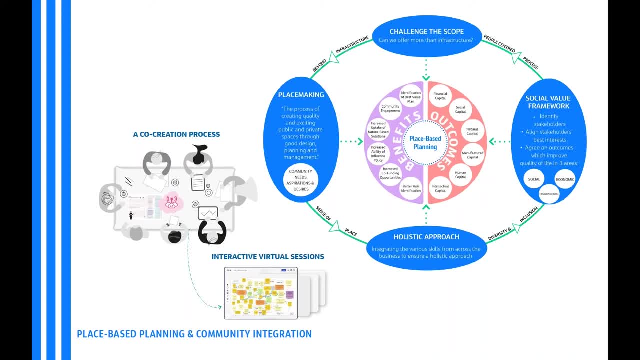 to play space planning, so thinking about that. every place is unique, so exploring community integration. so how can we co-design with the community and co-create the process and also the output of the process? so, as george mentioned the idea of challenging the scope and how can we offer modern infrastructure? so how can the infrastructure also? 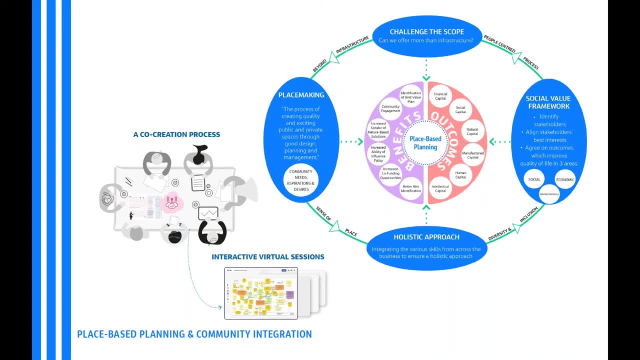 offer value to the community. so aligning the stakeholders best interest, which means like having outcomes that also improve quality of life, around social, economic and environmental benefits. so understanding these benefits and outcomes and how every project can deliver more uh through an holistic approach is how we have been engaging with clients. 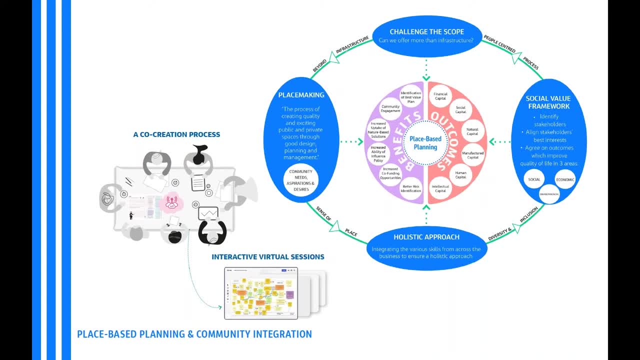 and delivering the projects. so we have been using digital tools for that. um, it was something that came uh during covet with the challenge of face-to-face workshops and engagement, which has been really useful, uh, because in the end i think that is not gladly we can face face meet again. but 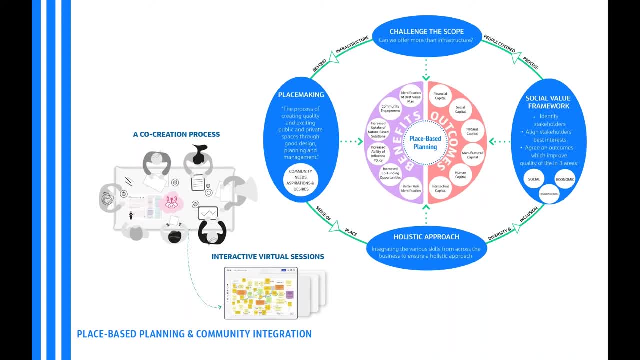 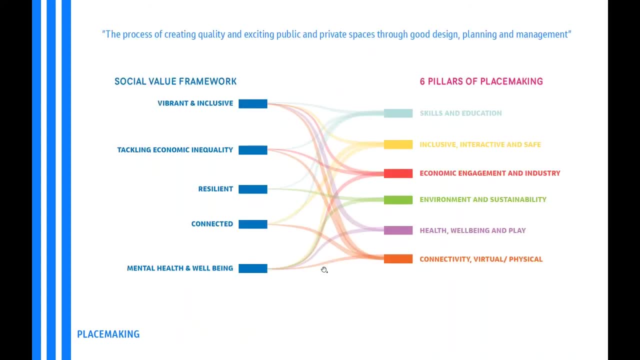 we can still explore digital tools to interact and engage with the community and with a wider range of stakeholders. so, um, the idea of place making, um, and it's sometimes not well clear to many of people. so we believe that place making is the process of creating quality public and private spaces. so how? 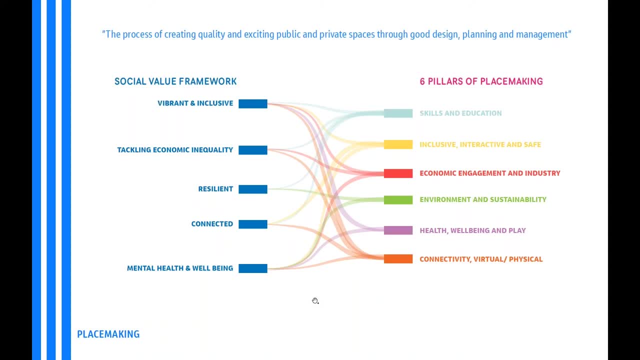 can good design, planning and management uh deliver quality spaces for the community and the social value framework um, um kind of sets um ideas around vibrant and inclusive places and tackling economic inequality and resilience, uh, and how place making can translate that into the public spaces. so we believe that the public and private space has the ability to deliver all this uh five uh. 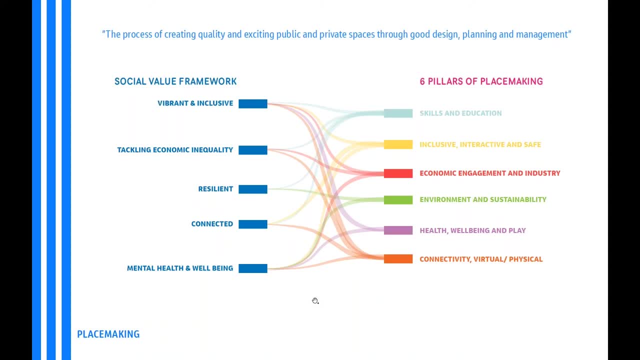 points of the social value framework when, when actually uh the spaces can be a place for economic engagement, uh, health and mb and play, and not all the kind of very traditional uh social value framework where where actually uh the spaces can act, be a place for economic engagement, uh, health and. 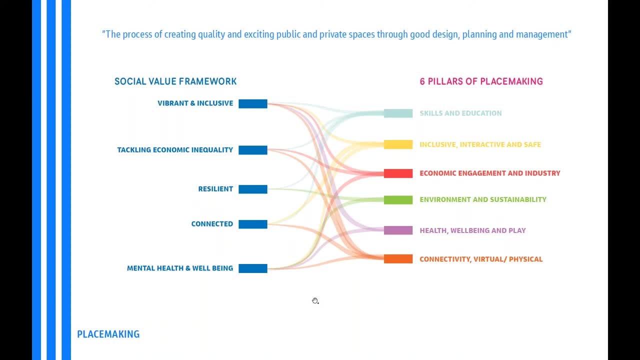 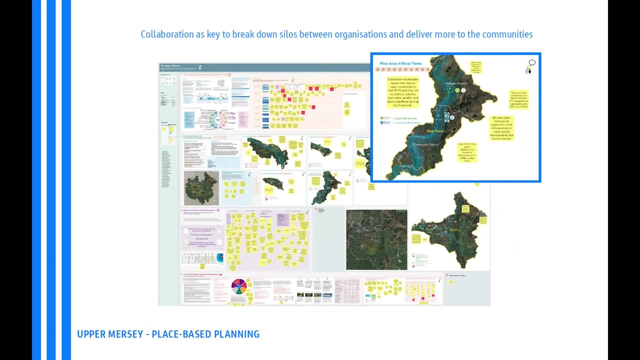 eb and play and not only um the mute folks's everyday activities but also other parts of the community, near the community and the only, as we expect, boring. So the Upper Mercy Playspace Planning is one of the pilot projects we have been engaging. we started engaging virtually and now we 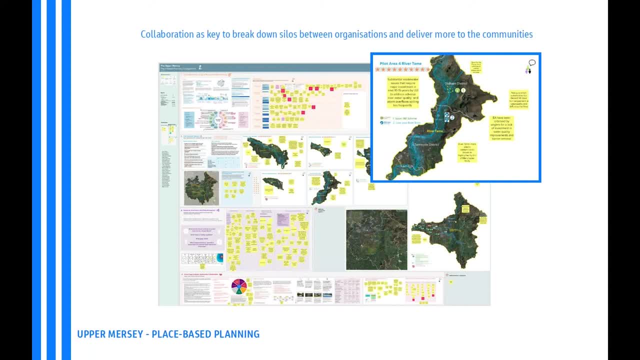 are started engaging face-to-face. So we use a tool called Mural, which is an online board where we can present to the clients and engage with the clients, and this project was basically a big challenge around breaking down the silos between the organizations, because when you look at the river, it's really 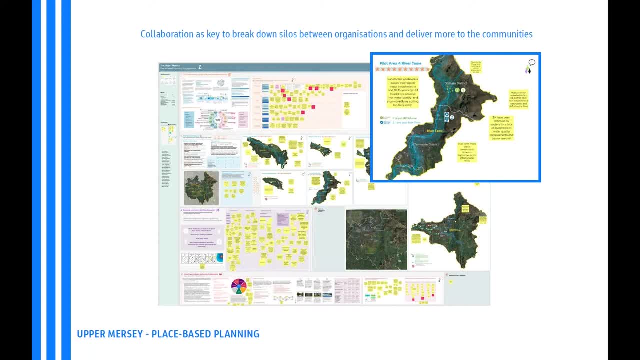 hard to define the boundaries. that makes local authorities, boundaries agencies, target areas and also the communities. So when you look at the upstream and downstream, projects have to be aligned, otherwise you're not delivering the best for that community. So the idea was to use this tool. 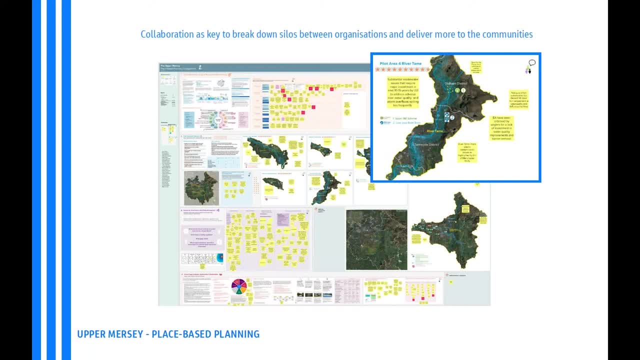 to engage online and it was really successful how people felt free to leave their opinion and their view of the issues around all the areas on the Upper Mercy and we are now piloting specific catchments within the Upper Mercy and engaging with the starting, engaging with a wider group to keep understanding more. 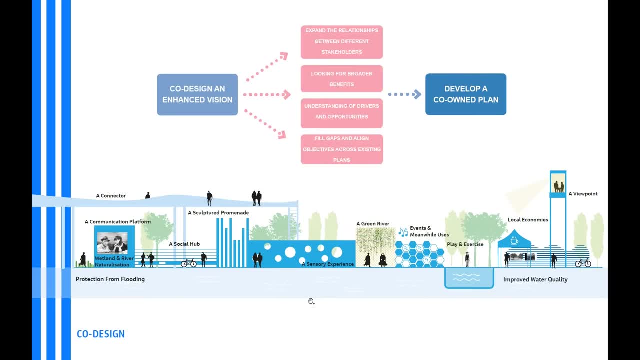 and more. how can we deliver more than infrastructure And this process? in the Upper Mercy, it's looking into co-designation in all the steps of the way. So, as I mentioned, about breaking down the silos, so in a way of understanding the drivers and opportunities and fill the gaps and 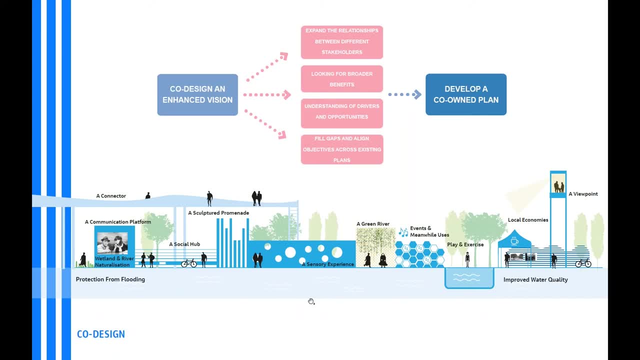 aligned objectives across these stakeholders groups, because sometimes people are doing the same thing and they are not communicating. so when you put everyone in the same group and they can see clearly how can they deliver more and not only thinking about protecting from flooding and improving water quality, but actually delivering places that can engage in directly with 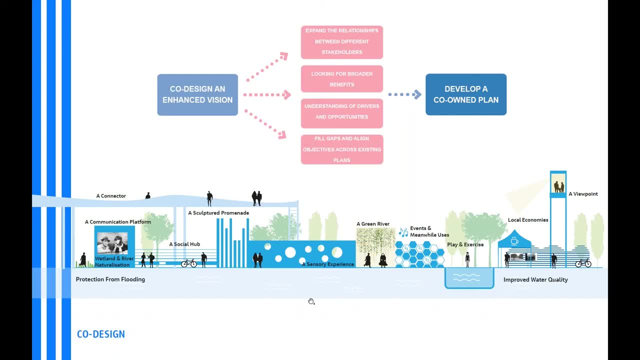 the community, and the community starts seeing the water as an asset, So creating interesting spaces. that involves play and exercise, social hubs, promenades and sensory experience where water is seen differently. We are exploring this with benchmarking examples to explain to the group how can we offer more. 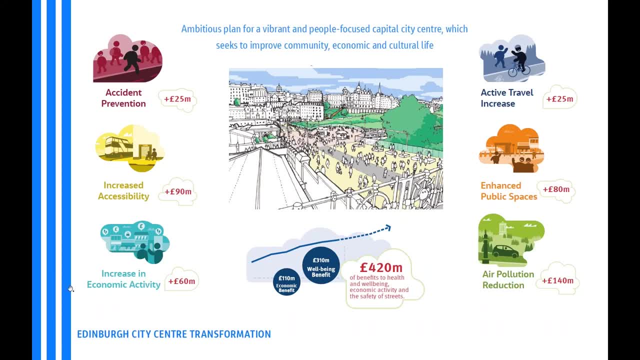 Yeah. so in terms of working with the government's social value model and I'm trying to translate into spatial principles, clients are asking: how can we measure really success? how do you measure these proposals against the framework? and really what it comes down to is the monetization of social benefit. 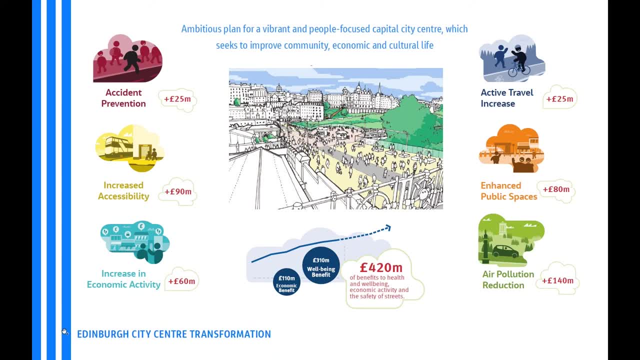 So this project example is in Edinburgh City Centre, which at the moment is fairly dominated by traffic, and it has fantastic assets: historic assets as well as cultural assets like the festival, with millions of visitors and tourists arriving each year, and the question was really, how can we switch to a more? 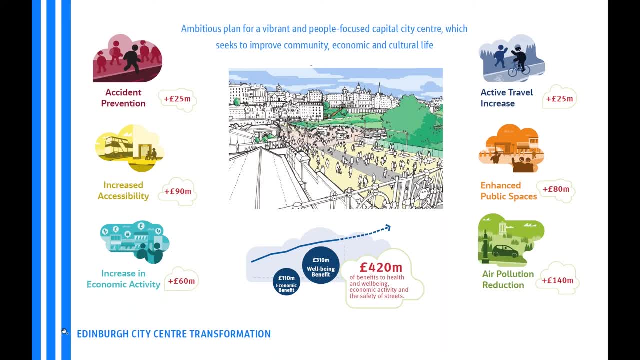 people-centric city centre, and how do we set those targets and deliver against them? and really by quantifying benefits against interventions. as you'll see on the side here, it becomes crystal clear and it's a language that's really important to understand. So I think it's important to 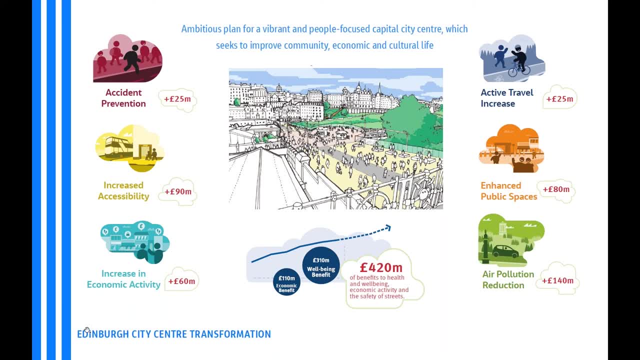 understand. So if you can say to them, we can show you how 420 million pounds worth of benefits will be delivered for health and well-being, economic activity and safety, that's something that nobody can argue with and the politicians are happy to stand up with and commit to. So this project really was a little bit of a. 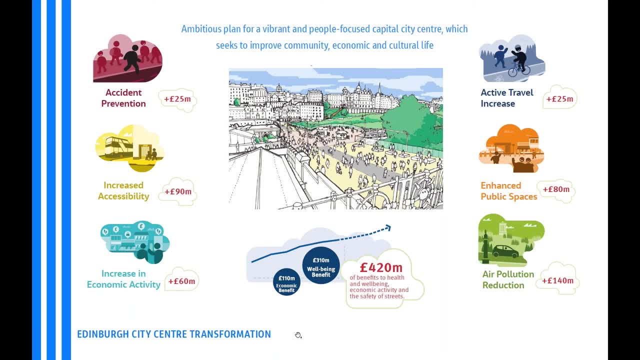 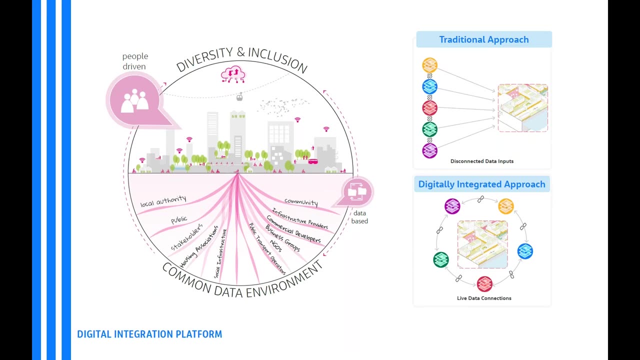 game-changer in terms of working with the council to set targets and then really set a roadmap for the future. So really, I think how we do this is to create a roadmap for how those targets can be delivered And in terms of how we work and how we collaborate as Priscilla. 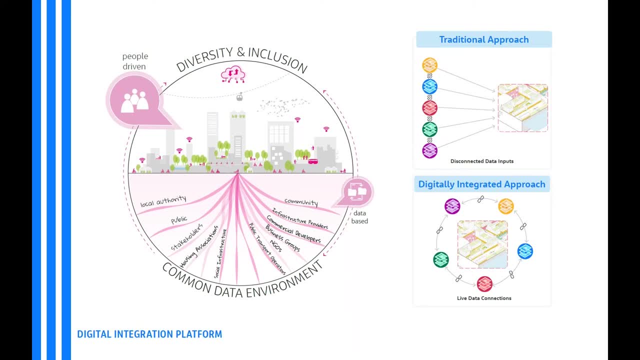 was saying, digital tools have become absolutely vital to that and in terms of delivering against a wide, wide range of objectives. as you see, on the left we see it as a way to integrate, to bring data together, to bring projects together with their neighbours and with the broader context. 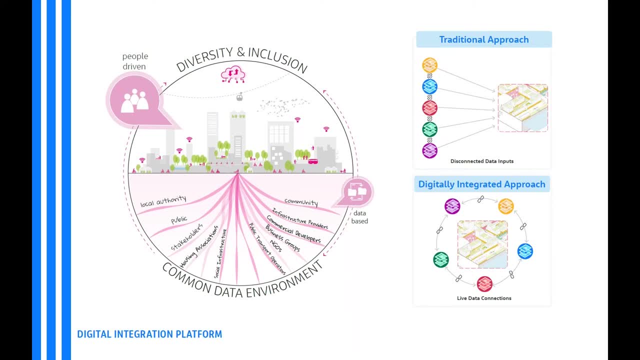 really demonstrate how projects are going to change places and change communities for the better. As you see on the right-hand side, traditionally numerous projects might happen in a place alongside one another, but not necessarily interact and would be carried out in silos. This digital integrated approach, which we call geodesign, is about creating one platform. 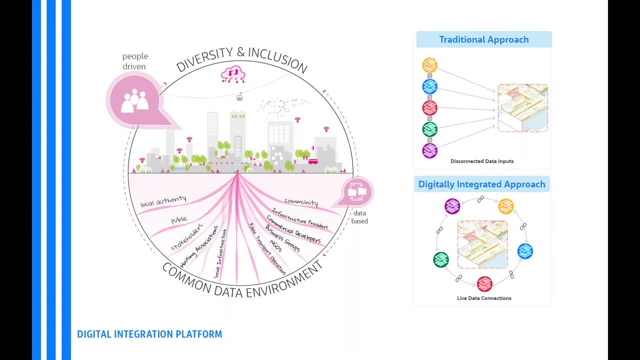 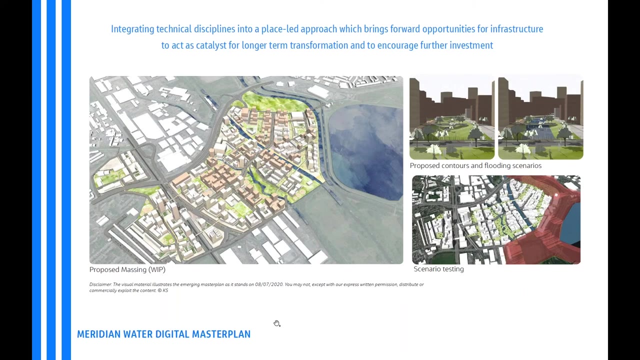 where everything can come together, be easily understood and allow decisions to be made within their context, not just within a silo. Meridian Water is the place where we've been testing this approach. Meridian Water is a huge development in North London which will 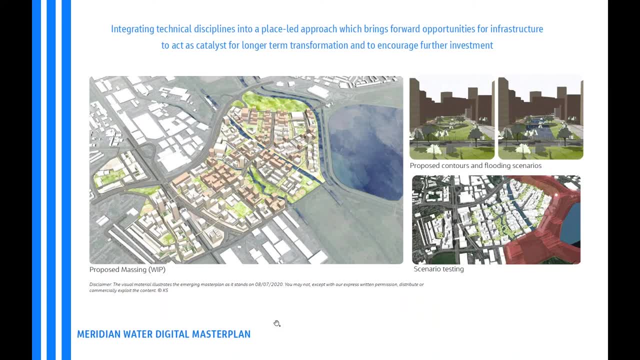 deliver around 10,000 to 12,000 new homes, 6,000 new jobs, and is, at the moment, a completely industrial site and quite a hostile environment. What we wanted to do was map the digital environment to change from now to 20 years' time, when the development would be completed and start. 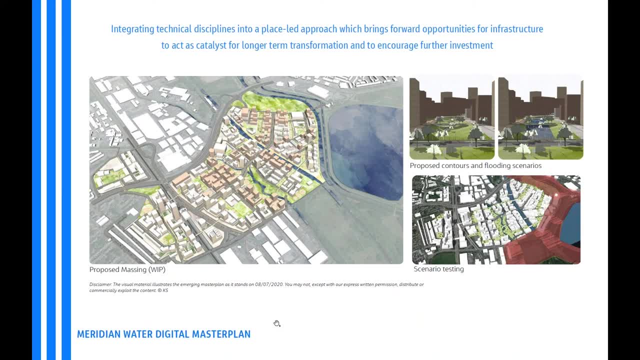 to look at scenarios for change. The geodesign approach really is perfect for scenario testing. You can use parametric software to make changes on the spot. You can demonstrate the impact of those changes environmentally, socially and economically. The project kicked off just as we were going into lockdown for COVID In terms of how we 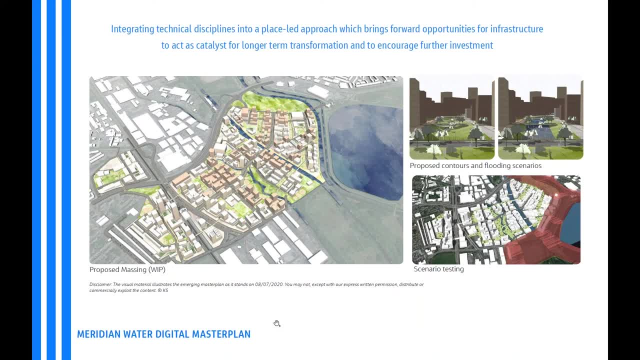 communicate how we collaborate. this was the perfect platform, really during COVID and really over the past two years, in terms of bringing together a design team across many companies, working with a council, with many departments, as well as other stakeholders and others who own parts of the site. 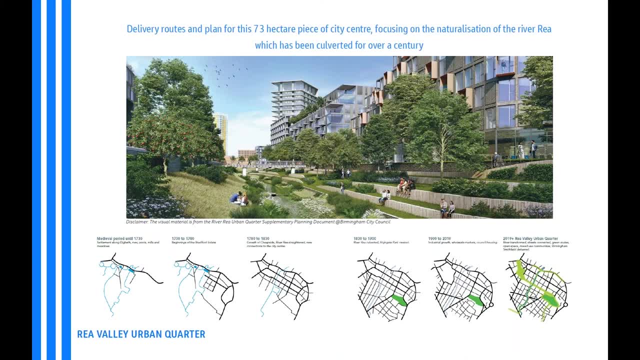 And River Ray Urban Quarters is another similar sort of project to Meridian Water. It's in the Bay of Islands. It's in the Bay of Islands. It's in the Bay of Islands. It's in the Bay of Gillingham City Centre and currently has a culverted river which runs through a very 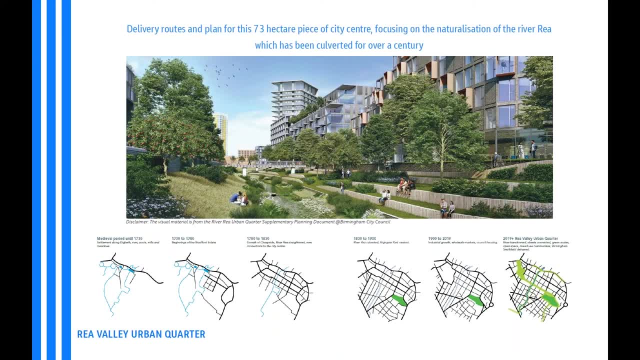 industrial part of the city And again we are mapping transformation from a very hostile environment to somewhere where people want to come and live, somewhere that can demonstrate positive influence on local communities, somewhere that can become a home really. And we again are using digital tools as a platform to collaborate, to work with the city, to work with 44,000. 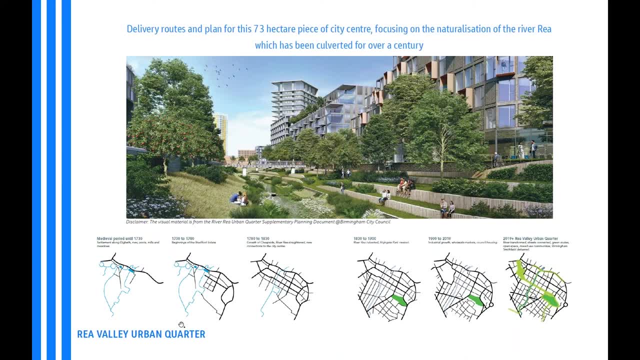 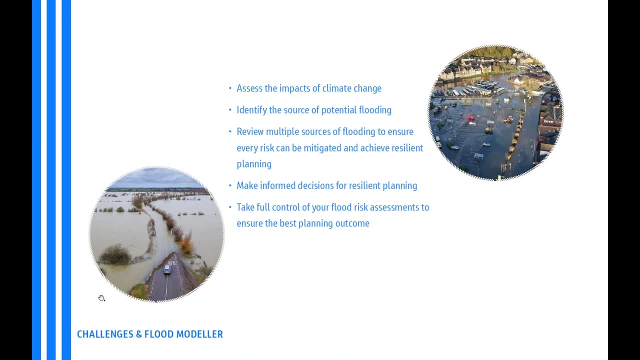 people, different stakeholders, and really map out challenges, risks but also opportunities, and set out a roadmap again over the coming 20 years which this project can be delivered. so the idea we have this presentation was to show how we have been working and how we have been trying to align different 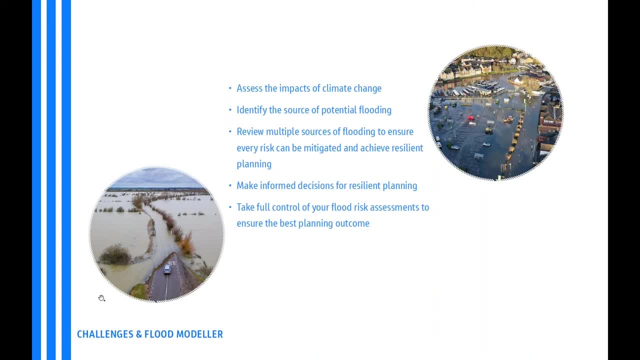 tools to deliver more to the clients and we think that the flood modeler is an amazing tool to assess this impact of climate change and flood is one of the biggest issues we are facing. so the projects that George mentioned, also some of the scenarios, and most of the scenarios changed accordingly to flood. 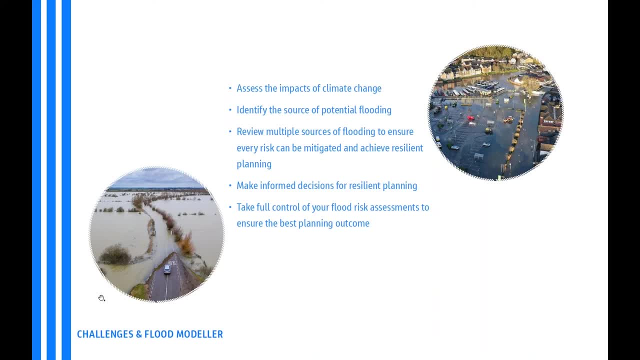 predictions for the next few years. so identifying the source of potential flooding is one of the tools that the flood modeler has, and also reviewing these multiple scenarios to see how they can be implemented in the future and sources to ensure that every risk can be mitigated, and also testing different 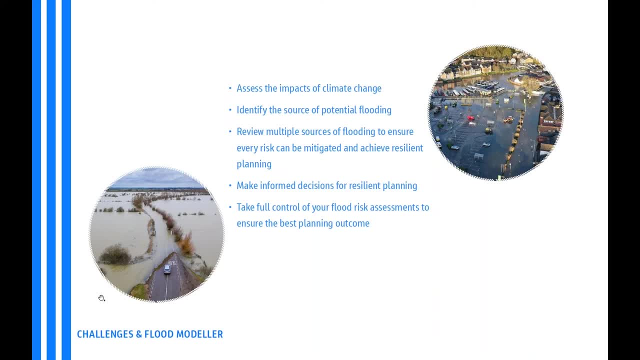 possibilities within the projects and so we can achieve resilience in planning and also think about all the things that can be tackled over time, so making informed decisions and also taking full control of assessments and ensuring that we have the best outcome. so I'll pass on to Mathieu to continue the presentation. 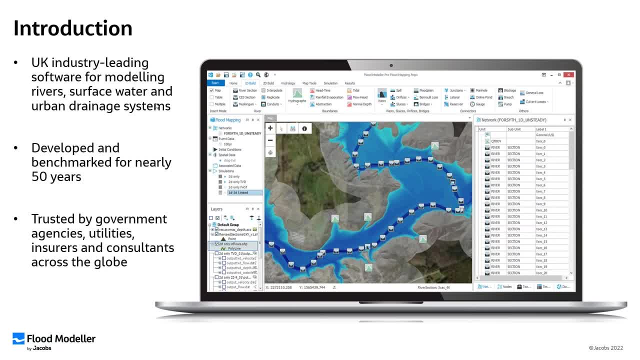 Thank You, Priscilla. so a quick introduction on what flood modeler is is the UK industry leading software for modeling rivers and surface water in urban drainage system is been developed by Jacobs and benchmark for nearly 50 years, is trusted by government agencies, utilities insurance and consultants across the globe, particularly the in the UK. here the Environment. 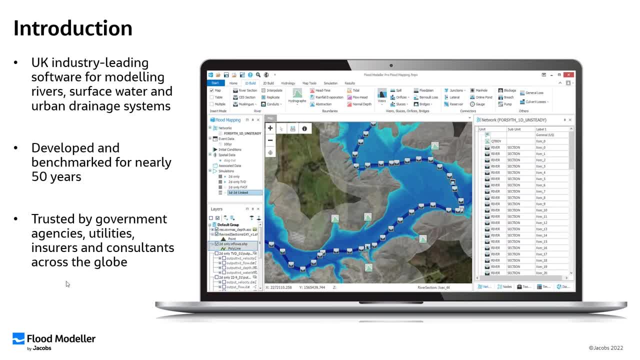 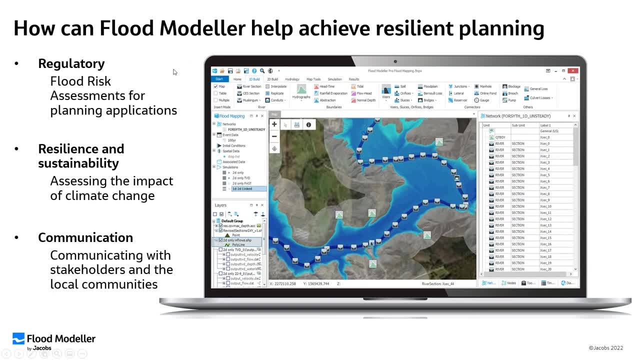 agency use it, as for national for forecasting, and is a key user of the software. so how can flood modeler help achieve resilient planning? i'm going to speak about three key items, once dealing with regulatory aspects, where we need flood risk assessment for planning application. uh discussing resilience and stability through the assessment of climate change. 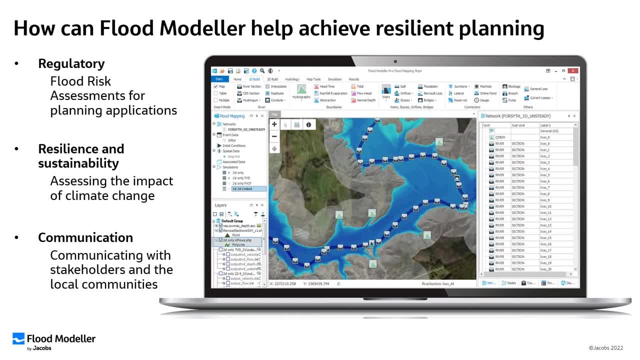 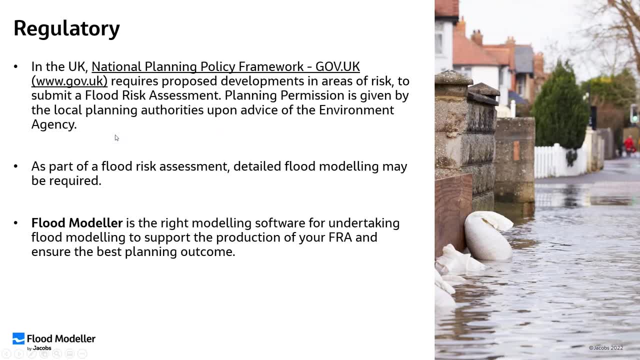 and how as well we can use flood monitor to communicate uh flood risk with stakeholders and local community. so to start with um, as you know, in the uk the national planning policy requires that proposed development in areas of risk uh requires so to submit the flood risk assessment and the 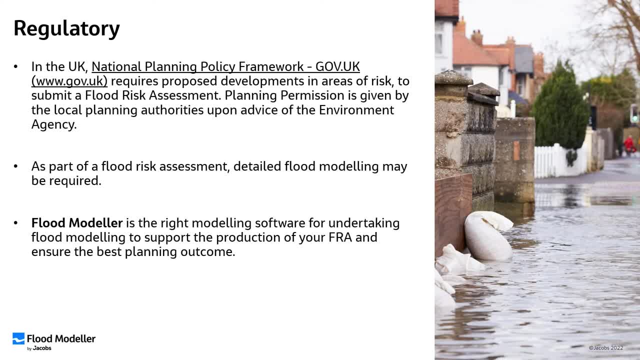 planning permission is usually granted by local planning authorities upon stature advice of the agent environment agency. a lot of the time, the flood risk assessment required detailed flood modeling and flood morale really is the right modeling software for undertaking flood modeling required to support the production of your fra. not only because of these capabilities. 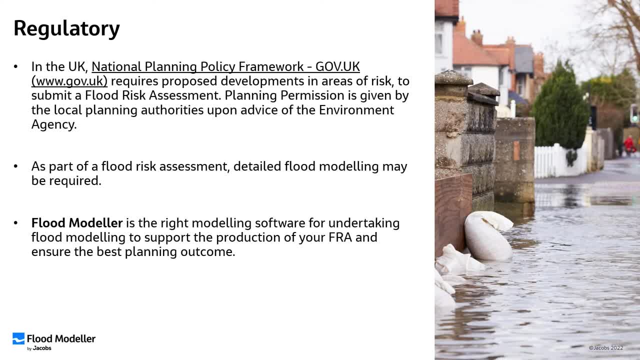 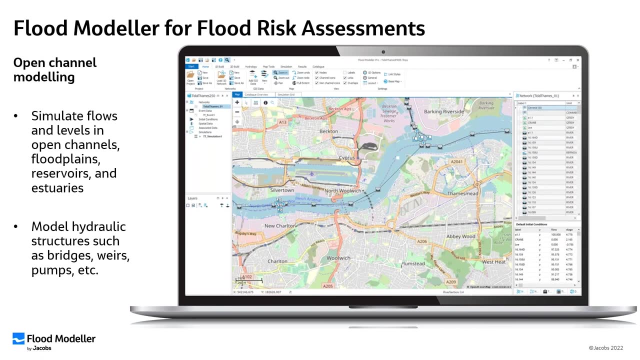 that we're going to show in the minute, but also as well, because you know this kind of project has been used and trusted by the environment agency, which can review uh, the hydraulic model you're going to produce to support your fra's. so, in terms of flood model capabilities, uh flood model can do open challenge modeling. 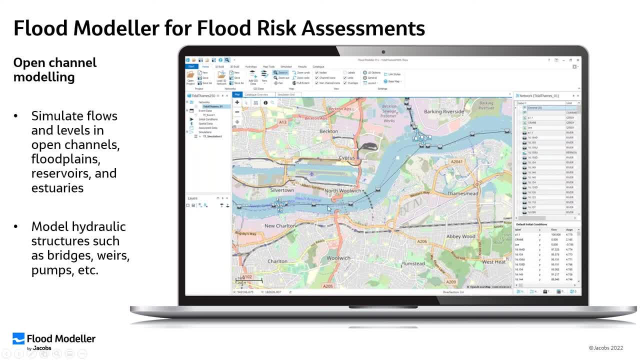 by simulating flood level in open channel. flood plain reservoir estuaries is accounting for any structures you might have across your rivers, such as bridge with pump. It's very easy to use and to learn. as you can see, there is a single graphic user interface. 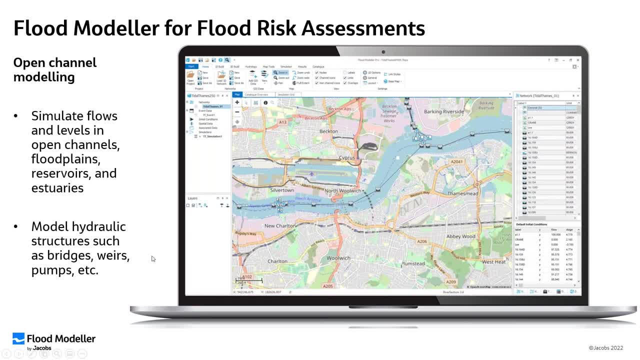 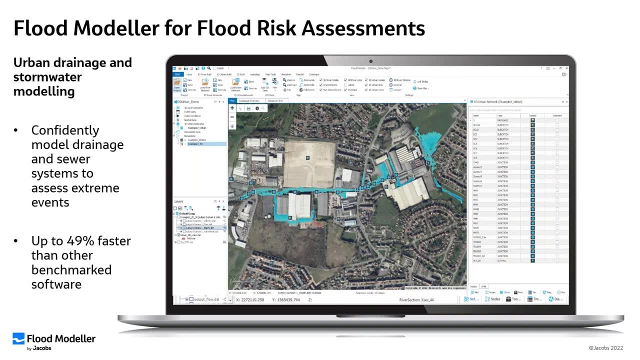 where you can not only build but also view your results. Flood modellers can do urban and drainage stormwater modelling. It can confidently model drainage and sewer system under extreme event. as you can see on the picture, there is when the sewer system is charged. flood modellers can model in your 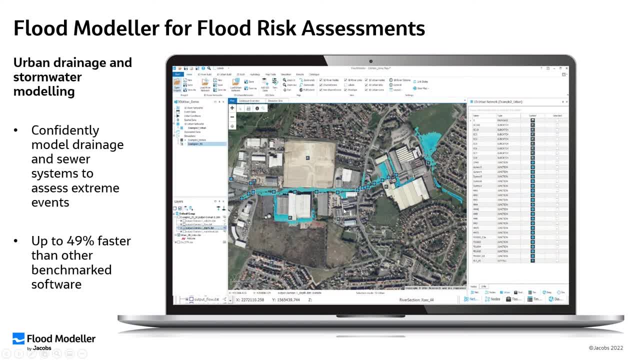 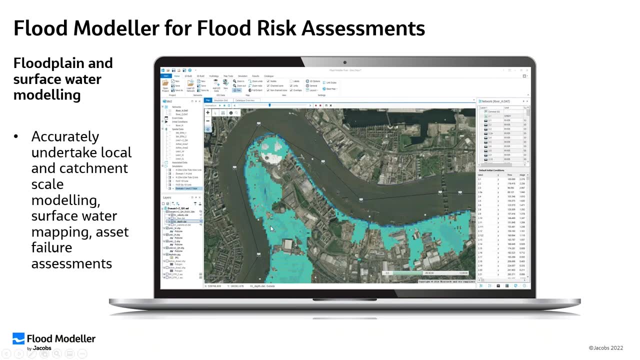 urban area, the excess of flow being routed by gravity. The solver flood modellers are very fast and usually 49% faster than other benchmark software. In addition for modelling urban sewer, you can do floodplain modelling, Such as looking at the impact of a failure of flood. difference any assets you've got. 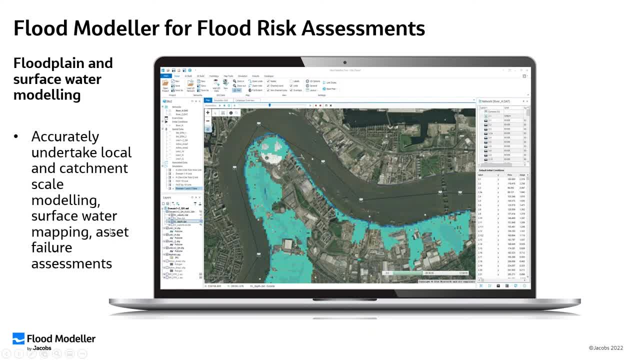 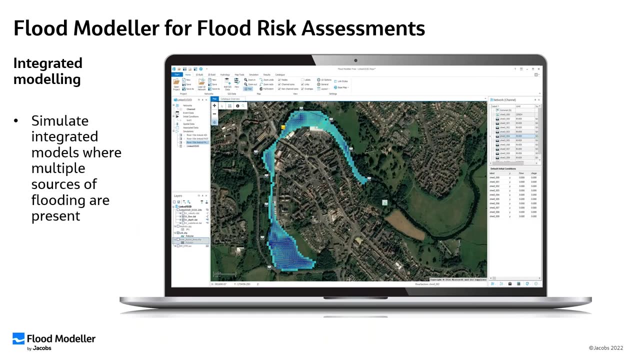 nearby your river, but also you can also assess the risk associated with pluvial flooding by using direct rainfall modelling. And, finally, if the risk is such that there is multiple sources of flooding in place, flood modeller being a tool Which integrates the different elements, such as the river as a floodplain and also the 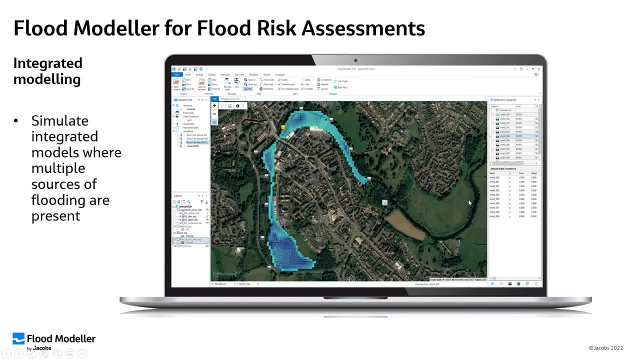 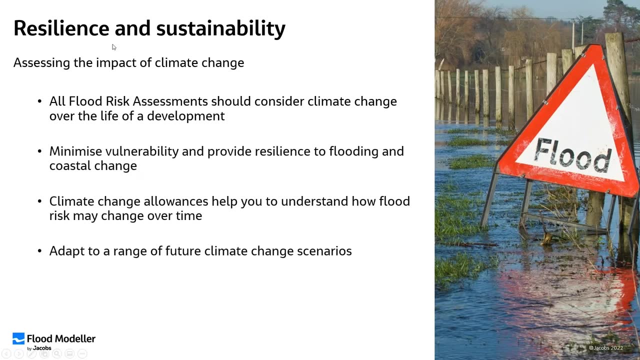 pluvial runoff, You can again using the single interface to build your model with, which require integrated elements. So the second aspect was around resilience and sustainability and the need to assess the impact of climate change. So this is a requirement as well for your flood risk assessment, because you want your 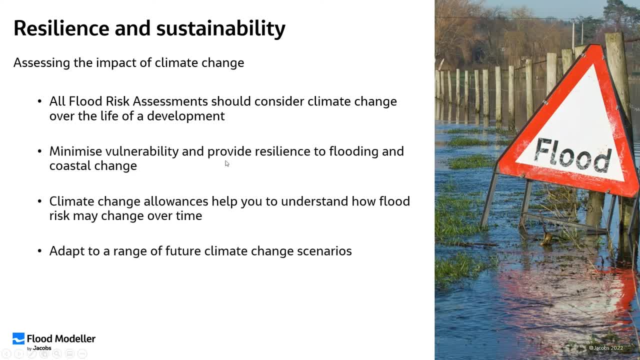 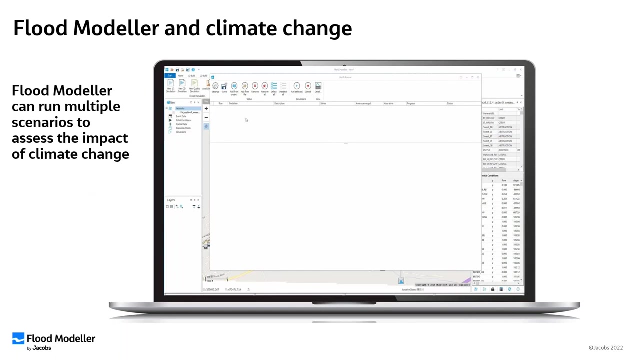 development to minimise the vulnerability and provide resilience to flooding under changes associated with climate change. So what that entails from a modelling point of view is that you often require to run multiple scenarios, Which, if you were to do it manually and one by one, it would take a lot of time. 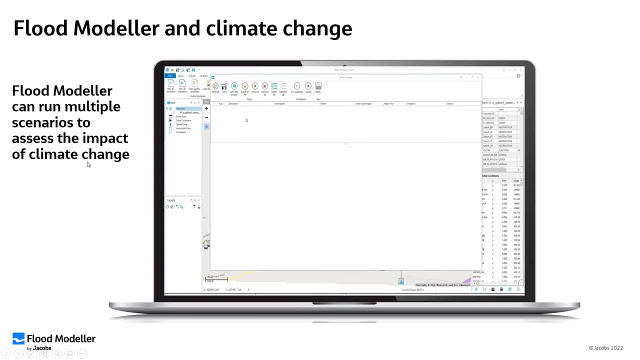 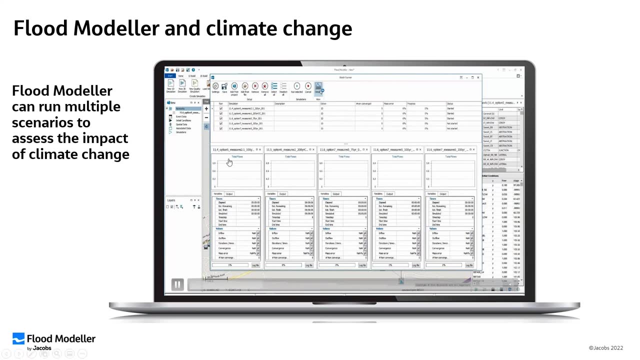 Again, flood modeller is really, really a right tool to do that and very easy to find. This little presentation animation is: show you how you can run concurrently different simulations to account for various scenarios associated with climate change. So you can run concurrently different simulations to account for various scenarios associated. 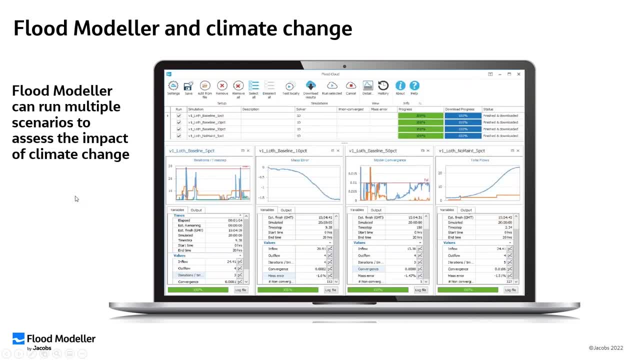 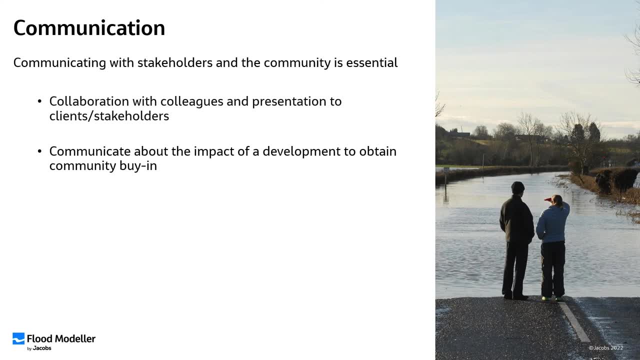 with climate change. Now, the last aspect was around communication. As we know, it's very important that we are able to communicate the risk to the people working with, as well as to our client, and also to get the community the local community. 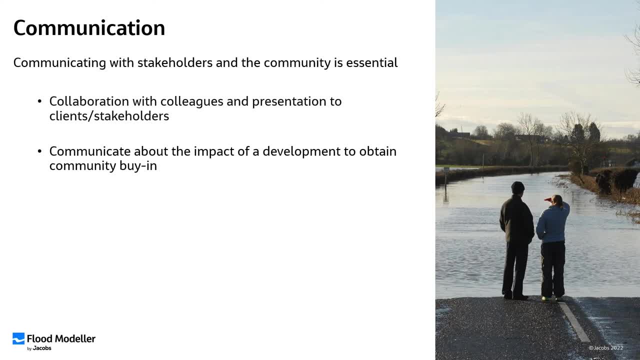 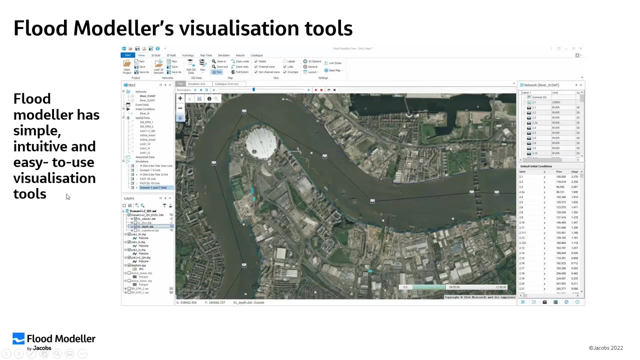 buying into your planning and seeing how your planning is going to be affecting or not the existing flood risk. So flood modeller has very simple, intuitive and easy to use visualisation tool. It's got automatic post-processing tool so that you can create meaningful flood maps. 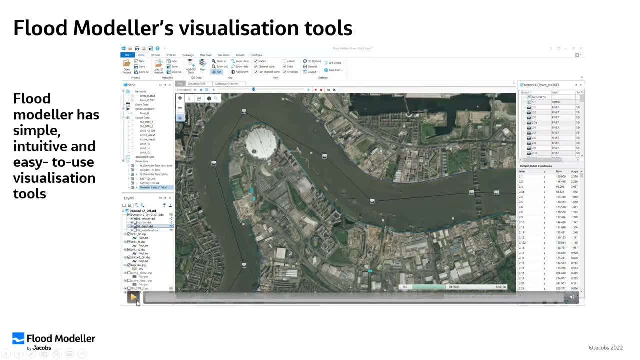 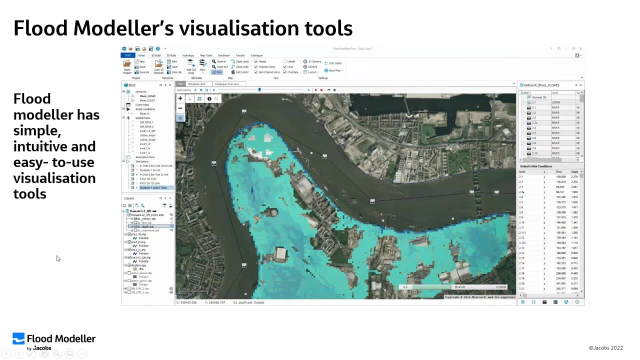 You can also see through this animation that you can, in the graphic interface, run, animate flooding and share that. This is possible by selecting the elements in the case that you want to use. So again, I'll be looking for examples in the next slides. but again, the flood rises. 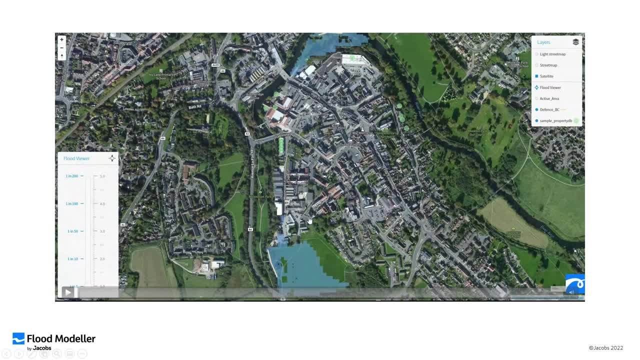 actually help you in secured disk space. So this is actually what you see is the flood moving on the site. So if you look at the vision and you can see there's a flood risk associated with this event, You can see this flood damage in previous slides. 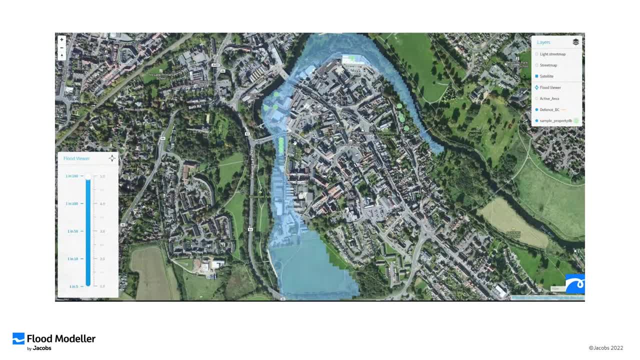 The low and the low. You can also see the flood risk associated with with with the flood events. So if you have a flood, what you can see here is that the flood risk is fairly high. So there's a lot of information about flood risk associated with those events. 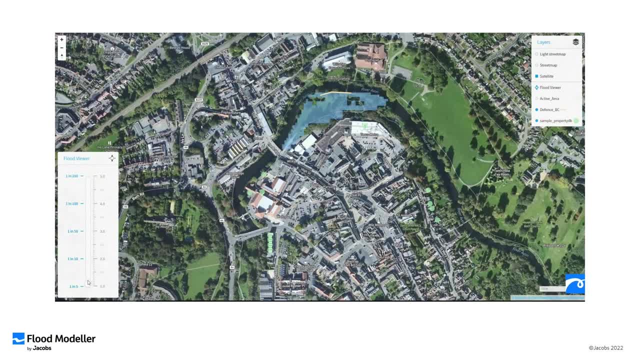 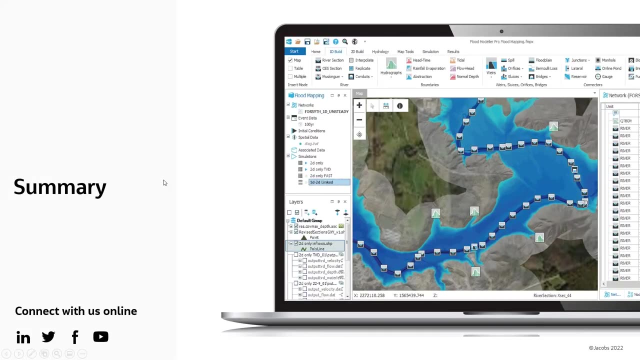 And then we can look at the and also, you know you can see on the slide, you know you can one in 211 and you can easily zoom where you want to see and represent the impact of your development. so, in summary, flood modeler is really intuitive to use, simple, it runs fast and is used by the. 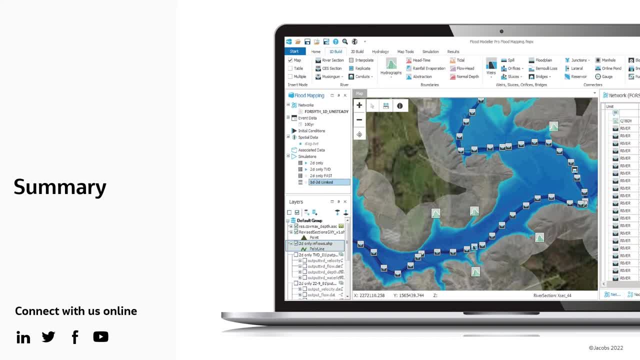 environment agency, which is the statutory regulator when it comes to some flood planning application. i hand it over now back to priscilla for concluding remarks. yeah, so it was a pleasure to present uh our work uh to you guys, and uh the idea was to mainly make it clear how we can work together and how important it is to test the scenarios. 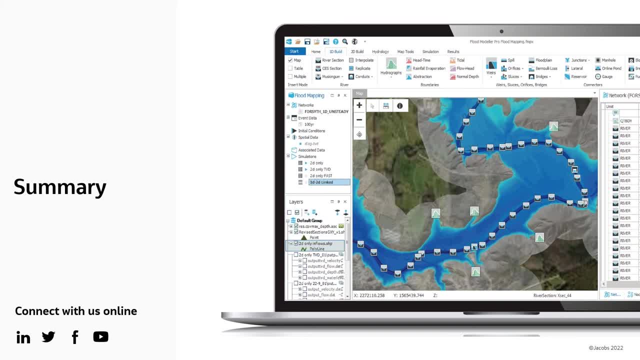 with flood modeler uh to help our work uh as planners, uh considering different scenarios and considering how things are changing quite quickly related to flood um. so we'd like to be open for questions and also, if you want to reach out to any of us through linkedin, through facebook. 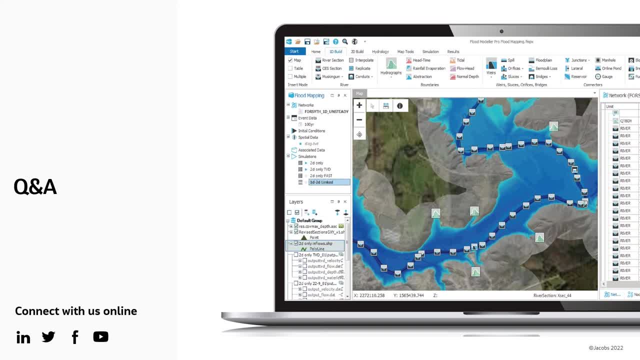 instagram, all the tools. we are happy to continue the conversation. and, yeah, marion questions. thank you very much. i was. it was really good, thank you. i hope um our attendees have found the presentations uh useful and interesting. um. we'll um move on to q a now. um so just give you a few. 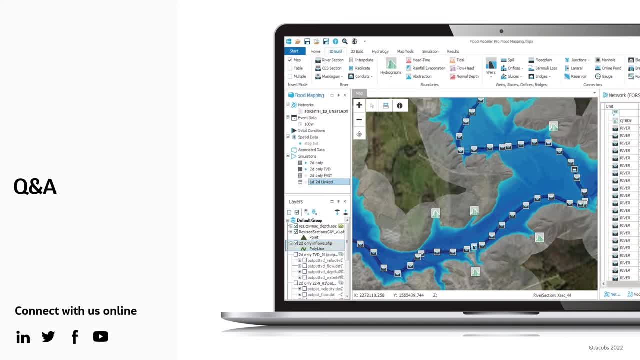 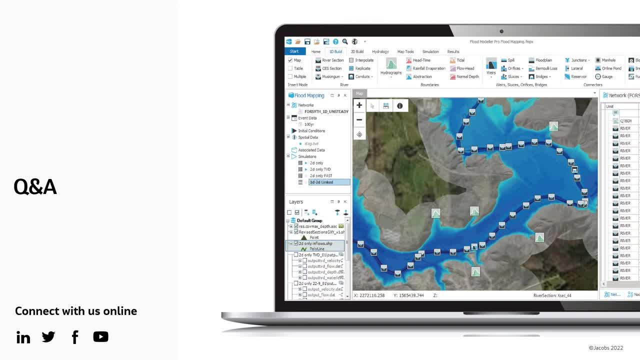 so, um, we will be in touch, definitely, right. so if i um look at some questions, so, um, right, so there's one. uh, actually, maybe maybe one for you. uh, priscilla. um, someone asked um. so during the design process, when should the flood modeling team start getting involved? 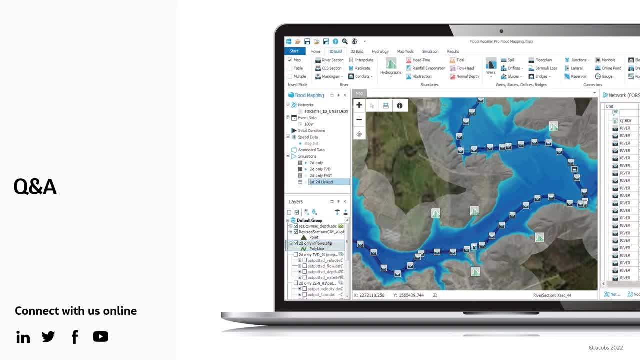 i think that it's a ideally it will be involved through different parts of the process so since the beginning, when you start testing different options at different scenarios, you can start analyzing the impact. so it actually informs the design since the the root of the idea, uh, and until 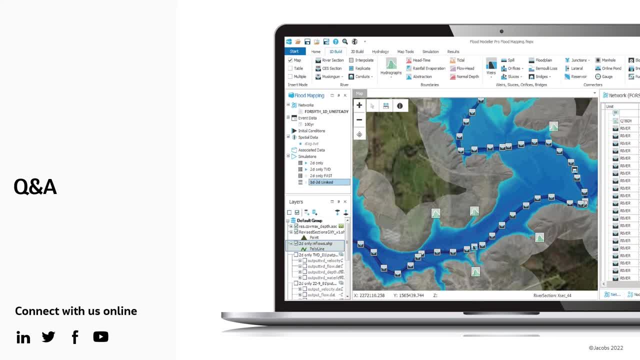 the end, when you start preparing assessments and and as the projects change and achieve the final process for planning. the assessments are, i think, really important to be part uh for planning applications and in overall assessments of how flooding will impact in the development. so, yeah, okay, thank you very much. okay, so next question. 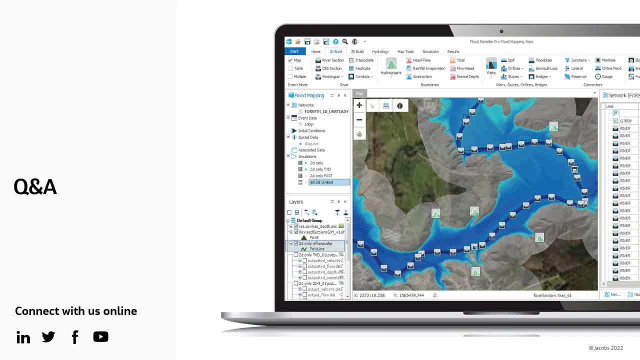 uh, maybe one for machio this time? um, so what climate change scenarios should be modeled and where can we find the data? so, most of the time, the- the climate change scenarios- is something that follow uh advice from uh the environment agency, and it really depends the region uh you are in, uh if uh, in particular, getting so you to to model the climate change. 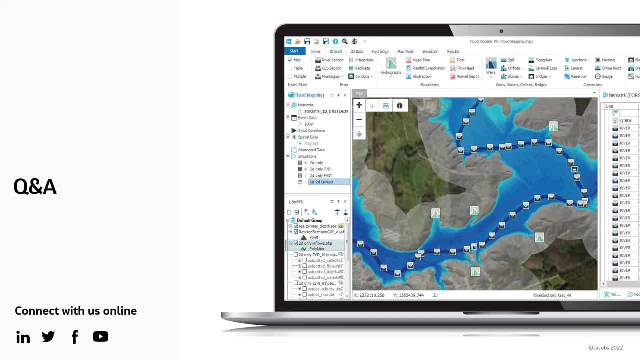 you would have to uh upscale the hydrological inflows going into your hydraulic model by a factor and to find out which factor you need to again deploy in the region you are in any guidance related to those factors available on a government website. i think on top of my head it's. 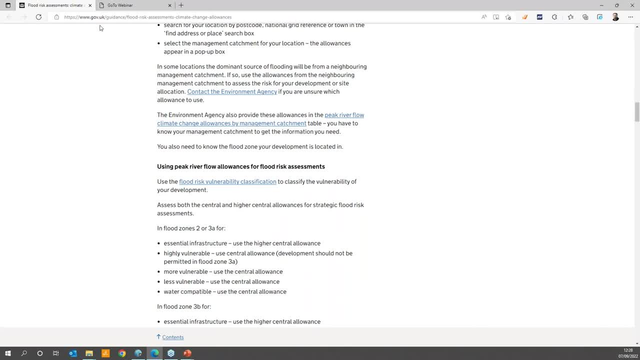 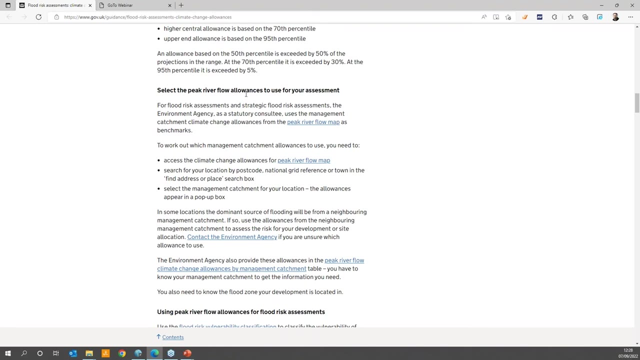 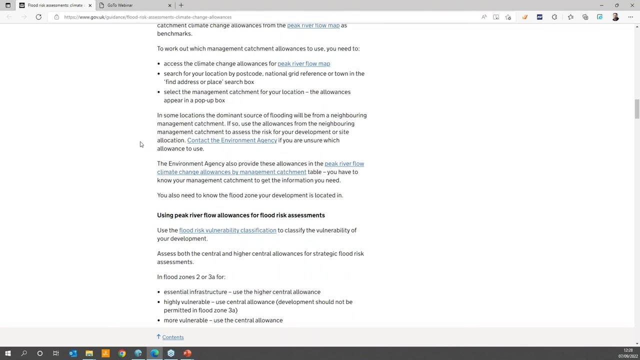 something you probably can see on the screen. it's on the government website related to flood risk assessment, and there is a very straightforward guidance in terms of feedback. uh, regarding the the data: the data is not uh completely new, and so you can see it in the website and you can see it in the climate change timeline. uh, in the data. 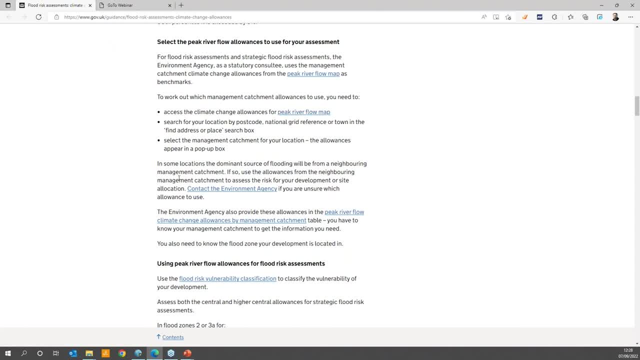 it's also available as a resource by the government, and so it's it's very useful for monitoring the data. it's also useful if you're learning about the danger of flooding. yeah, yeah, okay, thanks so much for the great presentation. thank you so much for your time. 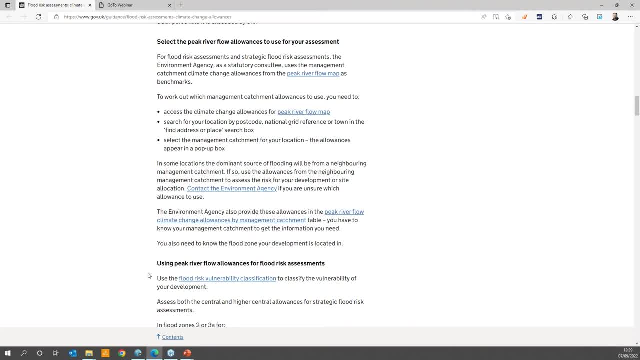 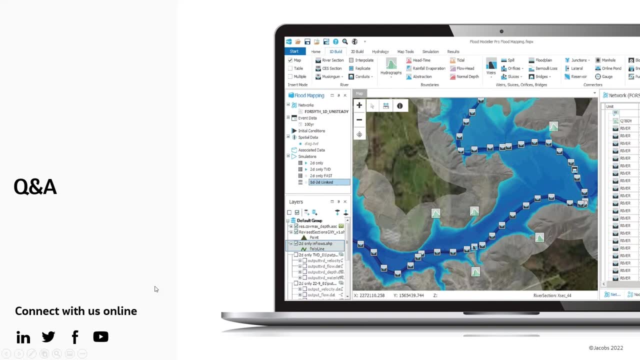 thank you, machio. that's great, really good resource, um, very useful, Okay, Another question, So this one may be for George or Priscilla. Someone asked how can flood assessment provide greater opportunity for regeneration or development? Yeah, I can take that question. So I think, yeah, having generally more accessibility. 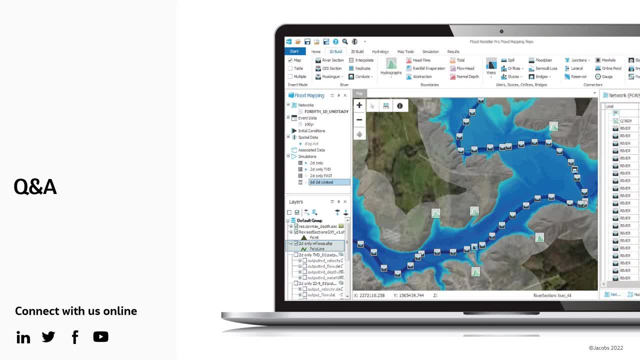 more transparency of flooding and the way that it impacts place is just incredible, I think, not only in terms of providing safety for existing communities and understanding of sort of future flood issues, but I think in terms of the pressure on delivery of housing within the UK and a lot of sites now disappearing and being developed. I think there'll be more and more. 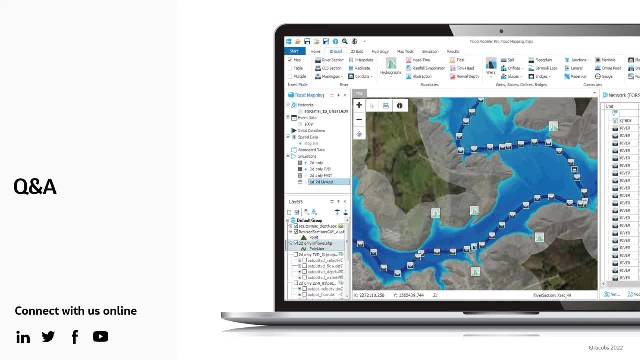 pressure to develop flood prone areas as we move forward, And I think having tools that allow you more accessibility, better visibility of constraints on those sites can only help speed up the process of development and regeneration, which is obviously a good thing. Thank you, George. Okay, So another question. I think this one will be again for Mathieu. 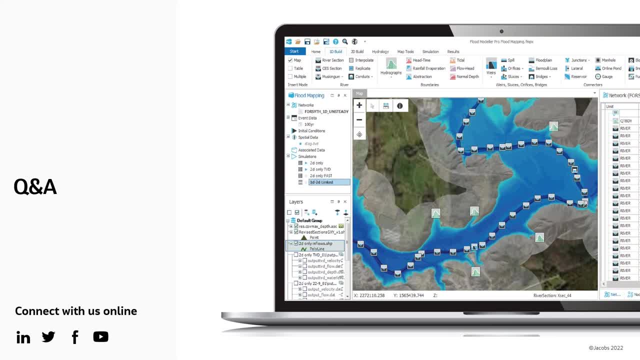 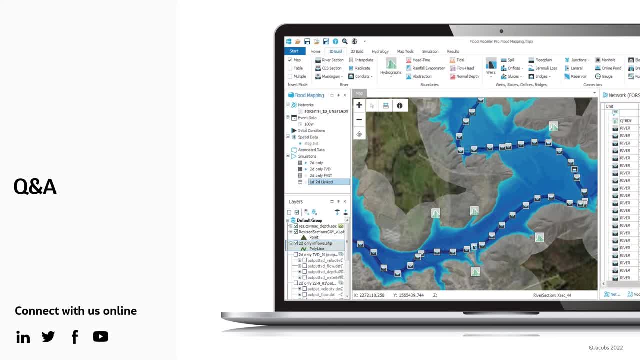 the assessment of climate change in estuary or near coast, you're going to need the guidance regarding the expected sea level rise associated with climate change. As demonstrated earlier, you can, with flood modeler produce, do floodplain hydraulics, So by simply applying a tidal bond. 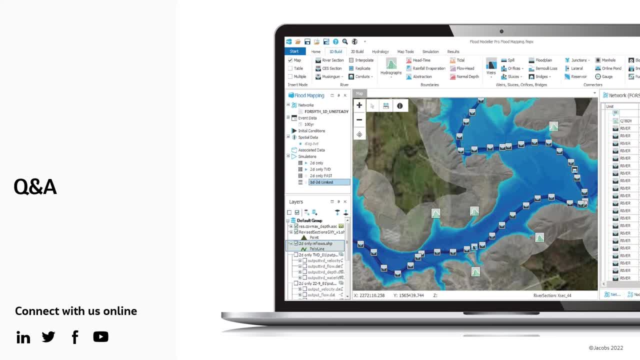 area which reflects the extreme levels that you would expect in the future. you can model the propagation of the tidal flood wave over the coast by all 2D solver. We've got GPU solver, which are the fastest on the market and they can easily under those kind of type of modeling. 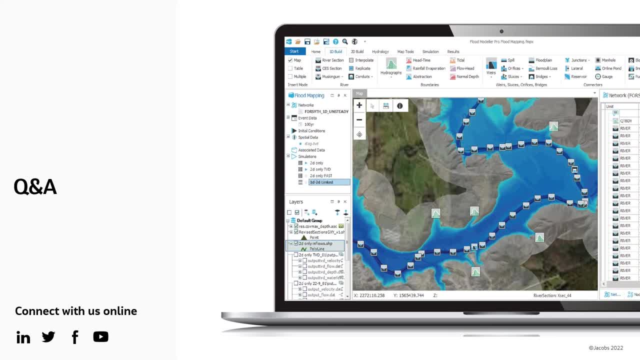 which is where very to request. Okay, Thank you, Mathieu. And someone asked about more information about flood modeler and about the software licensing and so on, So what I would advise is to just visit the website, so floodmodelercom. 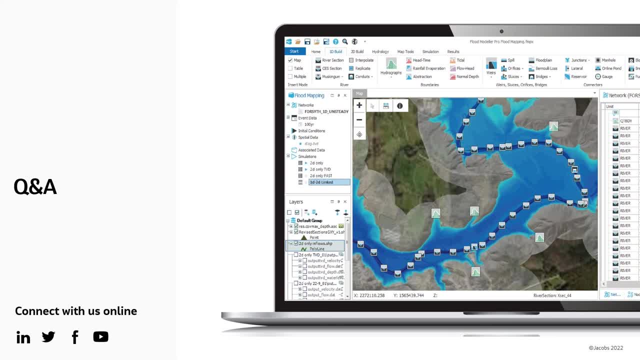 and all the information is available online And feel free to contact us as well. You can contact sales at floodmodelercom or training at floodmodelercom with more questions. And then I think we have a final question, I think again, one for Mathieu: quite a tech. 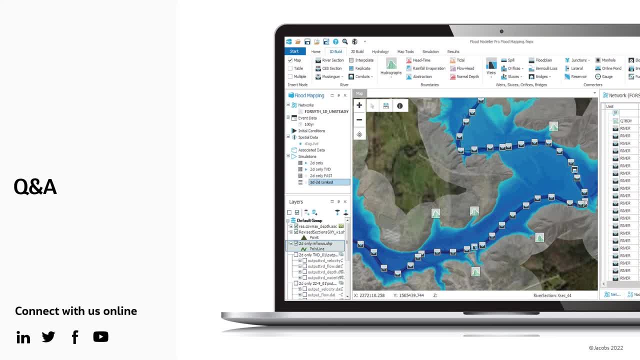 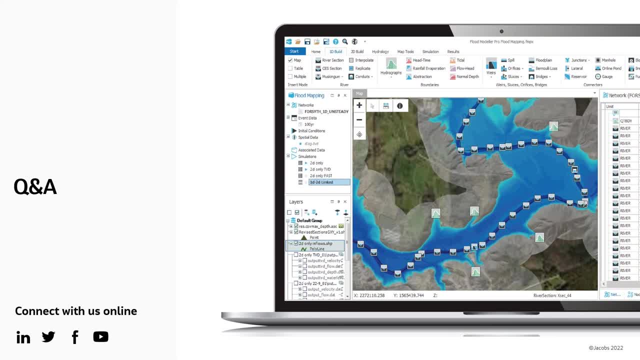 to model propagation of either a river overtopping its bank or, again, the sea through a tidal flow propagating. So you use what we calling a modeling, a two dimensional approach, where you're going to basically route a flow through the plan in two dimensional And the core information that you need to do. that would be obviously the 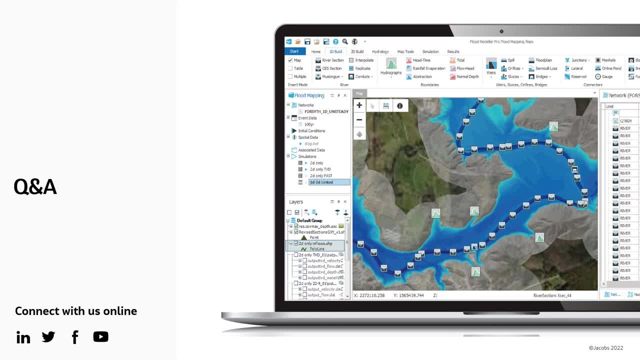 the topography of the land. We use very often in the UK and elsewhere in the world LIDAR data. So LIDAR data is obtained through aerial survey using laser telemetry and it's picked up at different resolutions. So you've got different LIDAR products. The usual one would be at one. 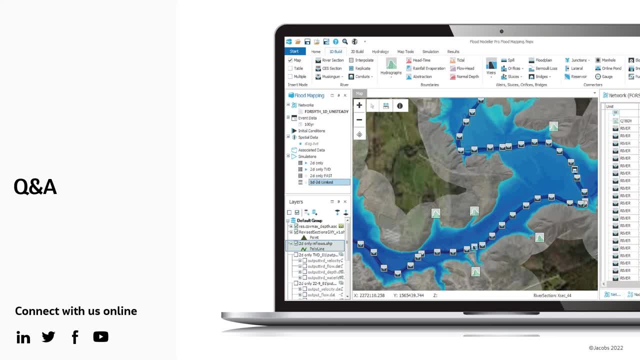 meter horizontal resolution to capture your ground level. but you've got LIDAR 0.25 meter resolution or a bit wider at two meter, But reasonably one to two meter would be enough to represent and to be used in your model For, you know, planning application. Now, one thing that needs to be the LIDAR and the topographic 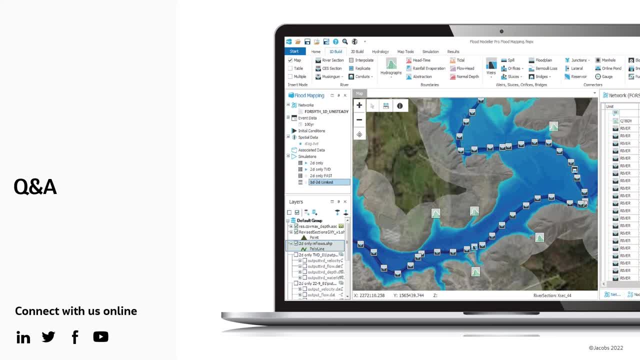 is one thing, but also, when you set up your 2D models, you set up which are based on what we call a feed, a fixed grid cell size, The grid cell with data in mind, the number of computation point that flood modeler will compute to return. 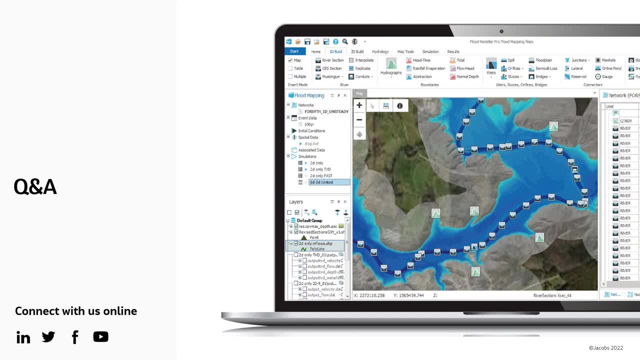 velocities and water level. So the grid cell size is going to be adjusted to the lens of how wide the land, the area he wants to represent, so that it's not too cumbersome to compute for the model. But thanks to the very fast and strong GPU solvers that we flood motor has, You can easily model up to. 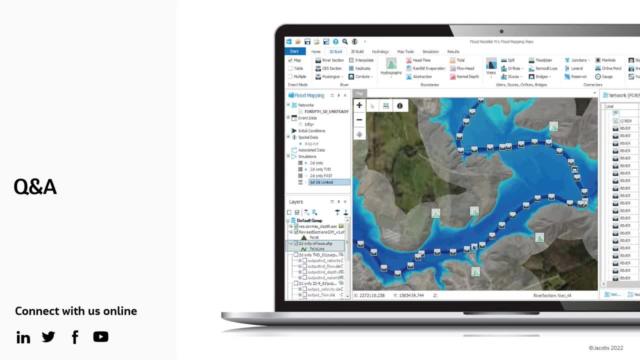 meter or four meter resolution in an urban environment where you want to model accurately the propagation of your floodways through the building, etc. Flood model can do that because we've got those strong GPU solvers that run very fast and give you an answer very quickly. 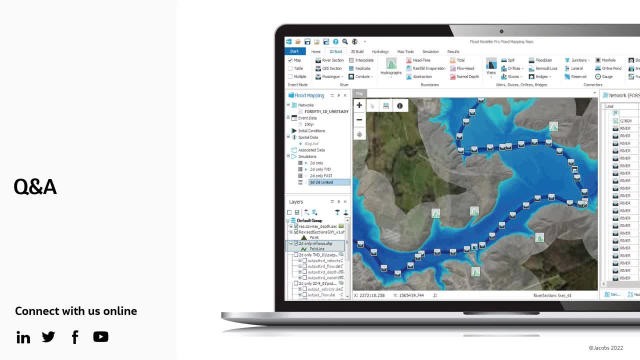 Thank you, Mathieu. It's a very thorough answer, Right? and last question is about flood defense schemes and basically, if I understand correctly, if we can use flood modular to design those flood defense or assess the strengths and going forward. Yeah, absolutely, We've seen that. 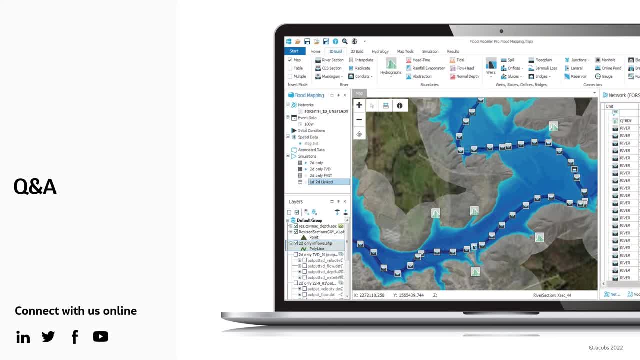 flood model has got the capability to represent open channels, so bank to bank, as well, well as representing in the 2D in an integrated fashion, the floodplain. So should you need to assess the effect of setting up linear flood defenses, you can. 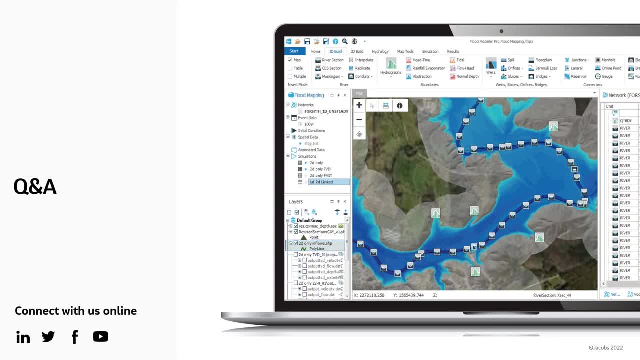 do that by saying: well, I'm going to build the baseline model of the existing situation and then I'm going to build another model, called a scenario model, with your flood defenses. Alternatively, if your scheme is based on providing storage- upstream storage- 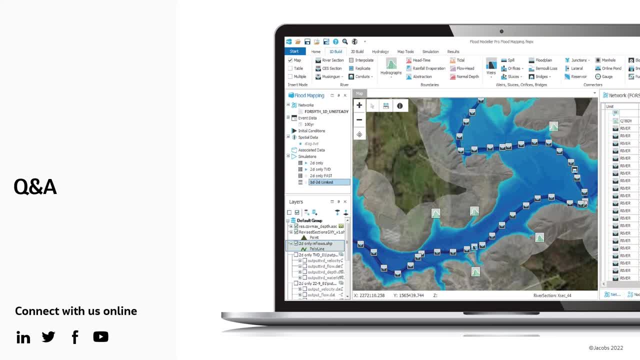 either online on the river or offline. you can do that by. if it's for online purposes, you can model a dam which is going to make the obstruction and the culverts, which controls the flows that are released downstream, to provide online attenuation. 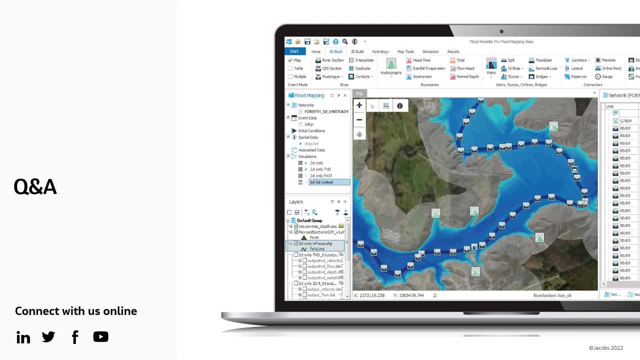 If it's offline, ie in the floodplain, you can carve in into your floodplain, which is with what we call a Z polygon feature, which is available in Flood Modeler, carving a depression area representing your storage area, And again rerun this scenario and assess the impact on. 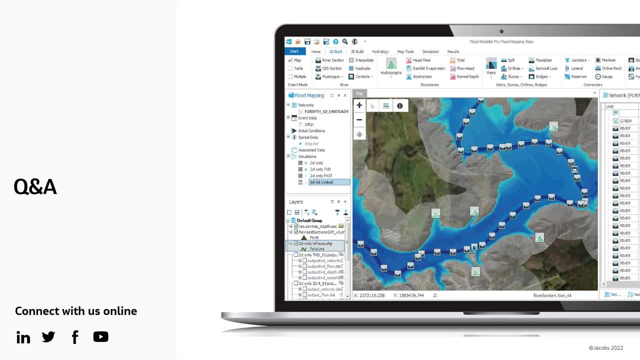 attenuating the floodway As you want- Perfect. Thank you very much. Okay, That's it for questions, So we'll do this webinar to a close. Thank you everyone.